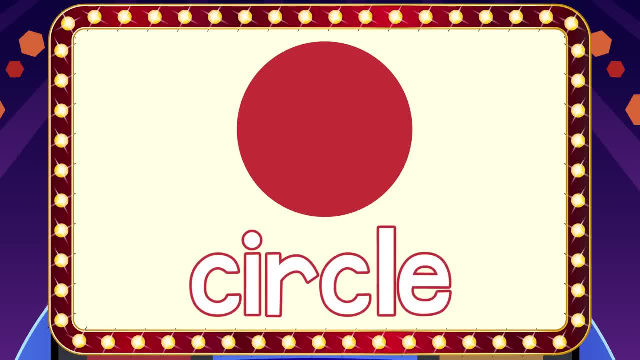 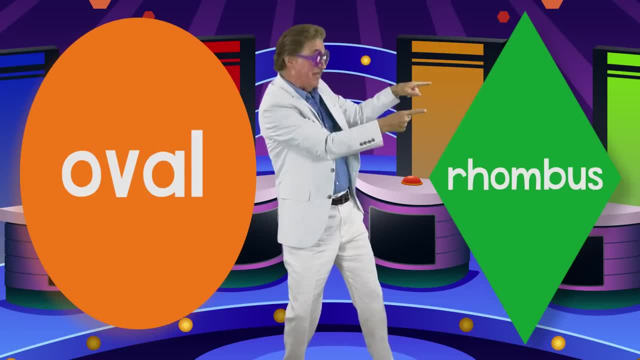 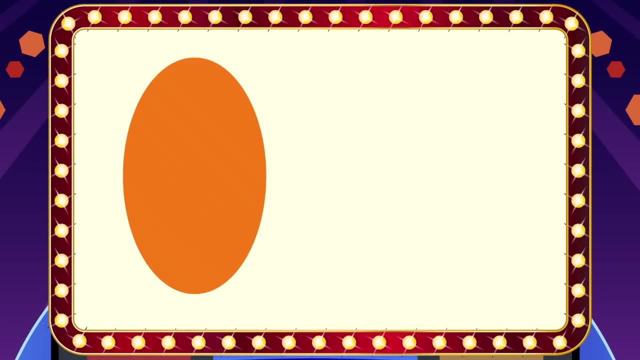 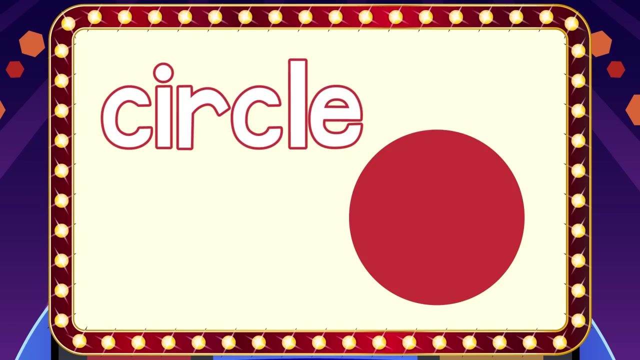 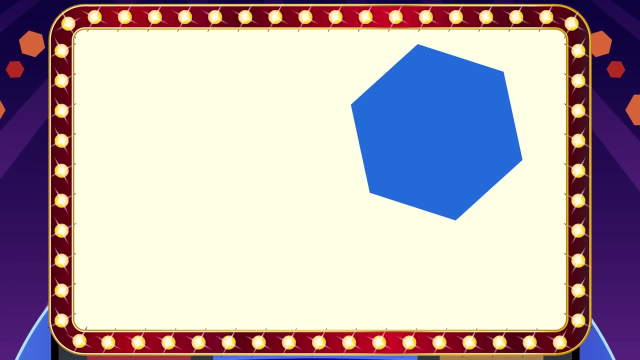 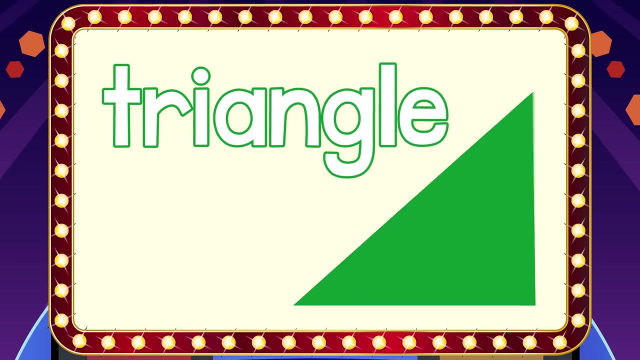 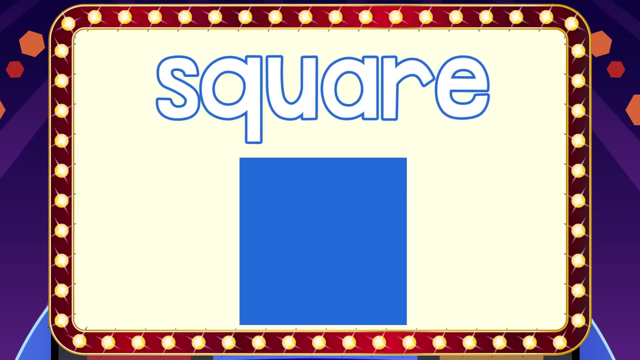 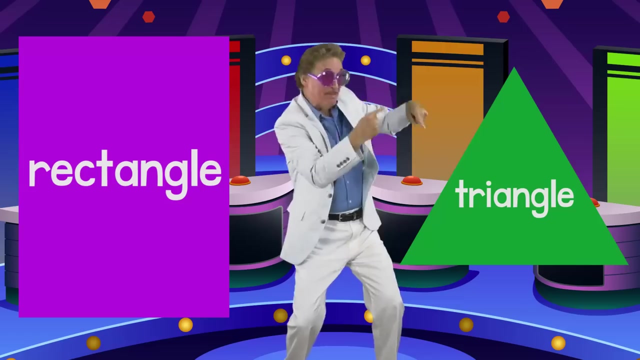 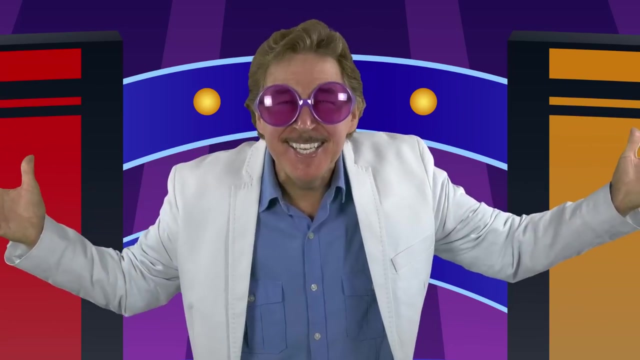 circle. name the shape game. It's fun. Name the shape game, Play everyone. square, oval, circle, rectangle, hexagon, triangle, rhombus, square. Name the shape game. It's fun. Name the shape game, Play everyone. Now you'll see the shapes in all different places. 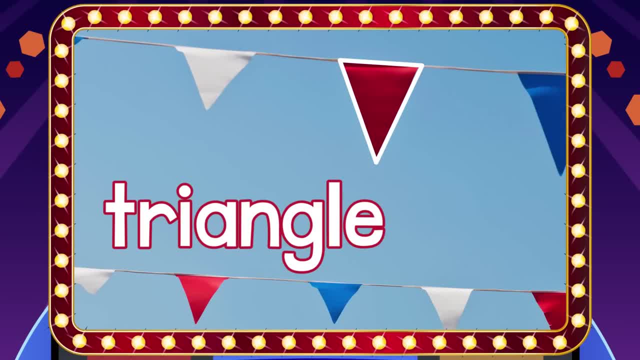 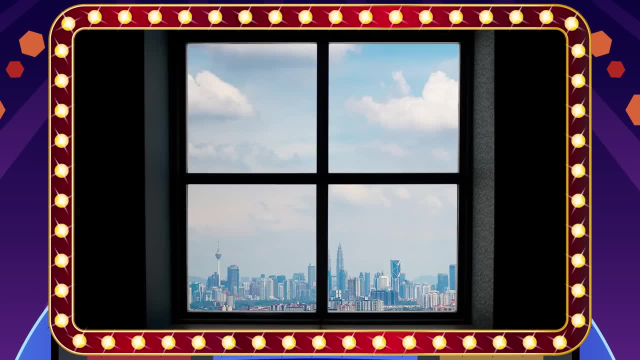 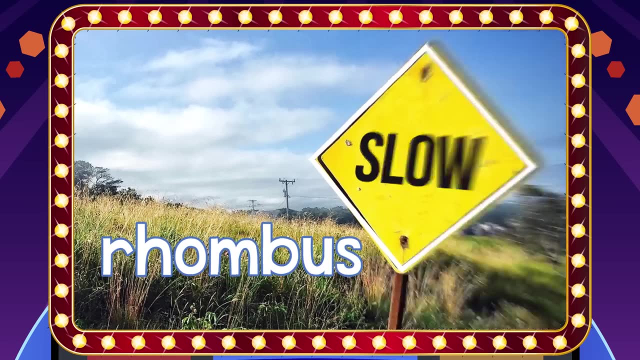 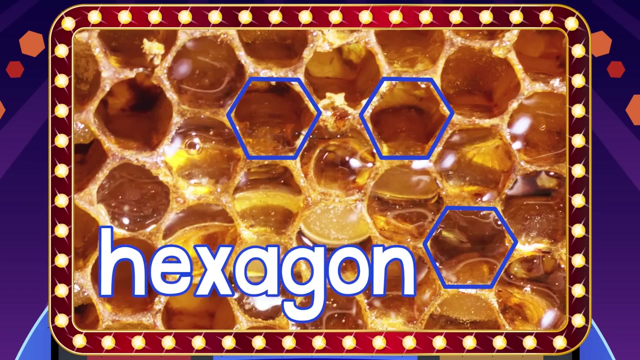 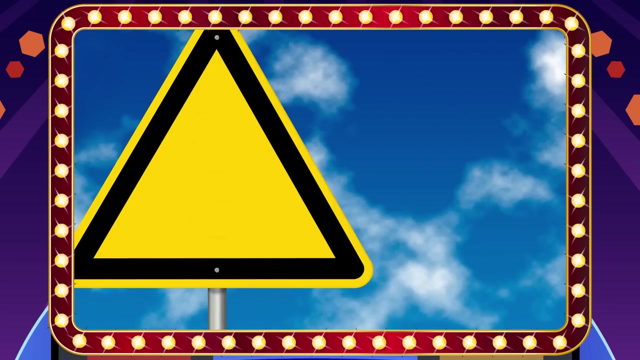 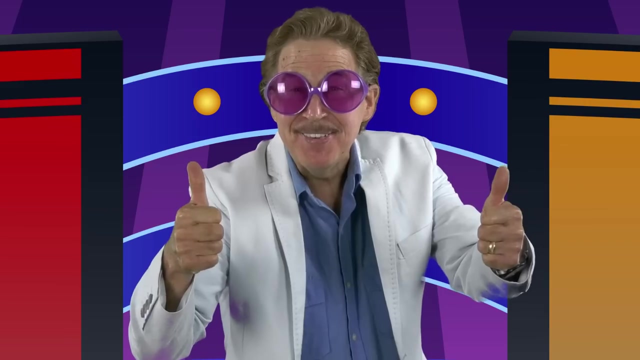 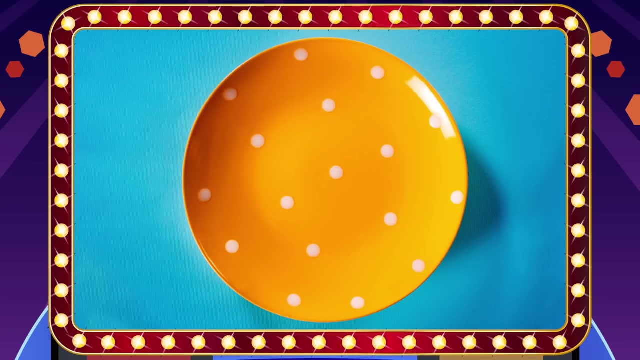 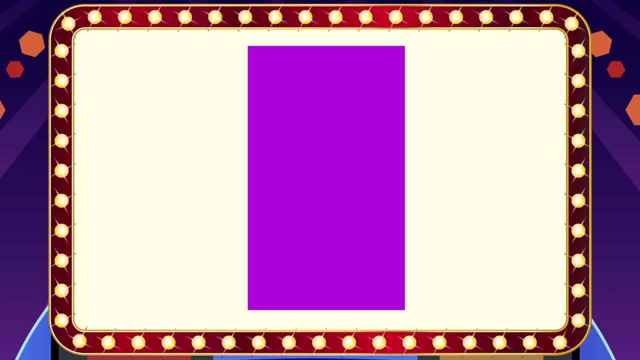 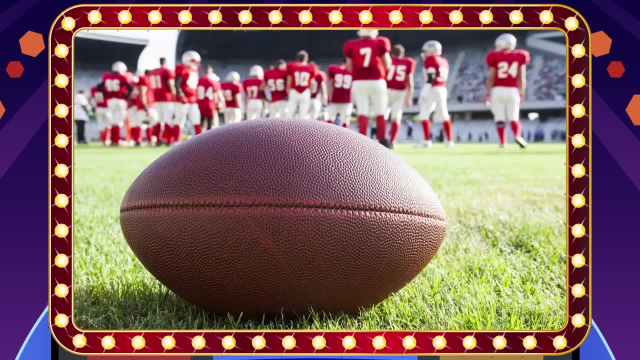 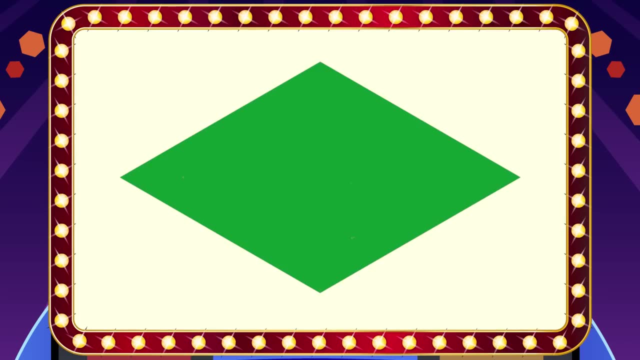 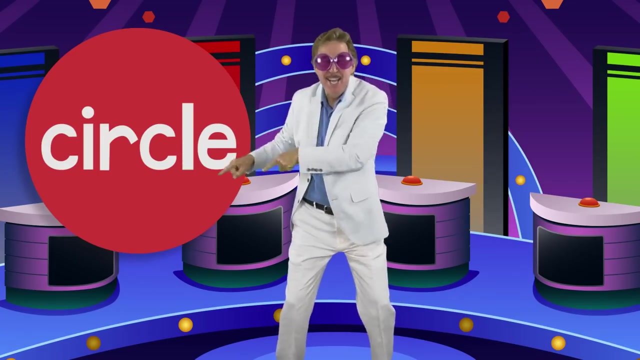 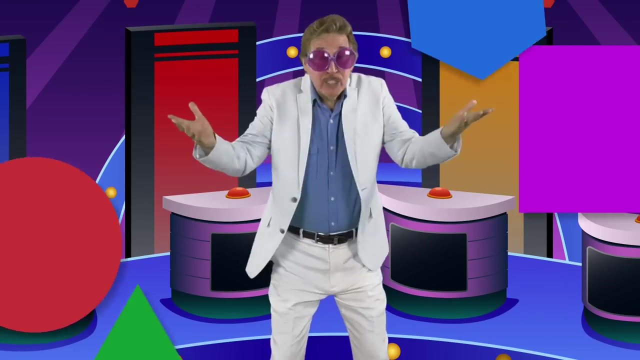 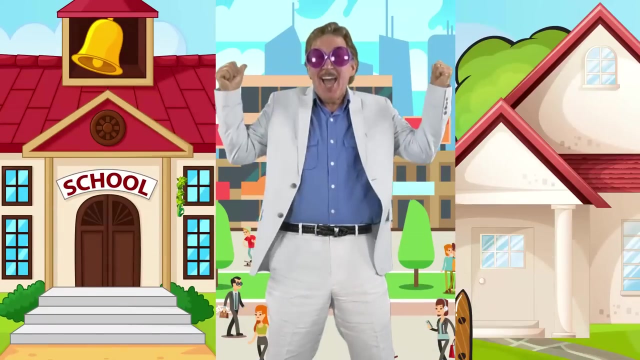 card expression. card expression: Name the shape game. it's fun. Name the shape game, play everyone. I know my shapes. I see them all around And you can see them too At your school, home or town.